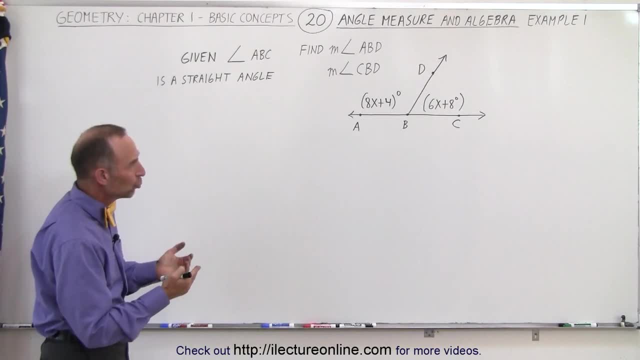 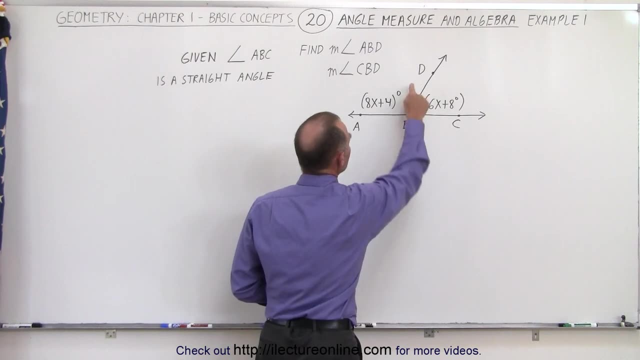 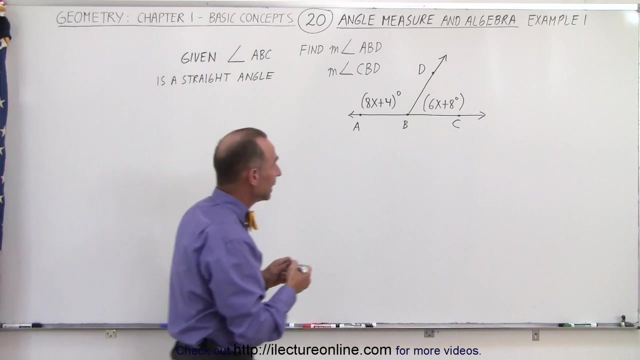 Welcome to our lecture online. Here we're given two angles. In essence, we're really given three angles. We have the angle ABD, the angle CBD and the angle ABC. So there's essentially three angles, but two of the angles are given the indication of an angle in terms of x, and I guess I should. 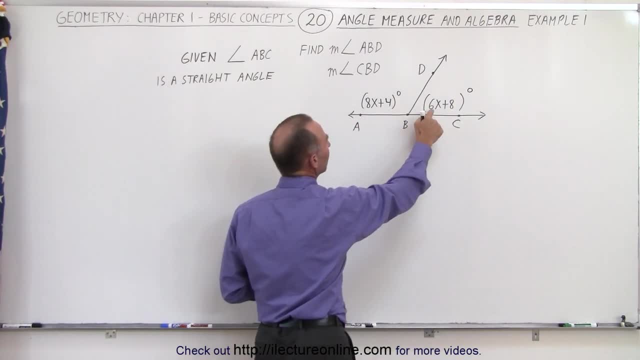 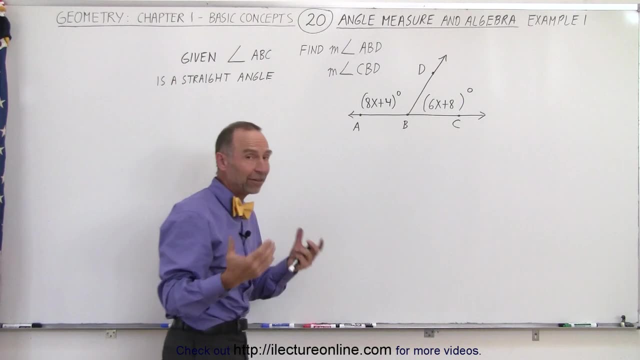 write it like this: We have 8x plus 4 degrees and 6x plus 8 degrees for the measure of the two angles, ABD and CBD. So now they're asking us to find the actual measure in terms of degrees, given that the 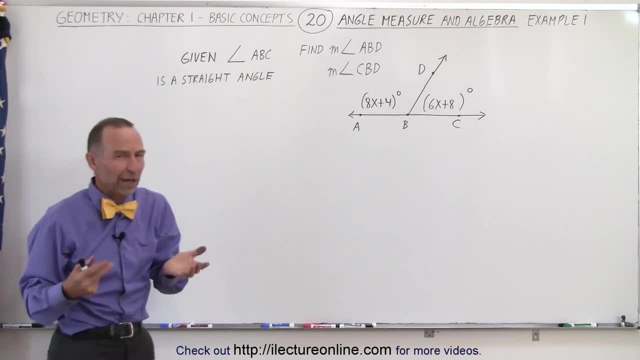 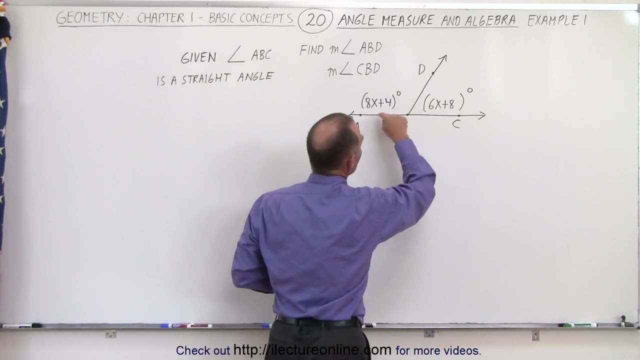 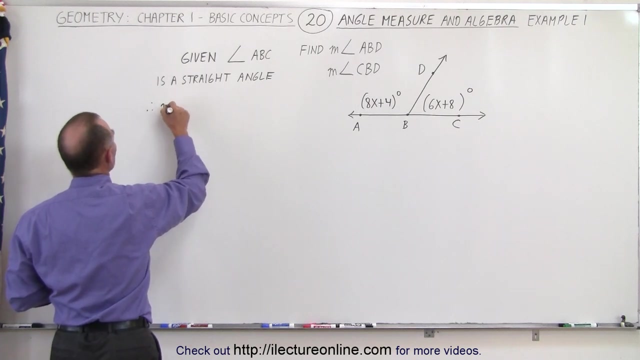 angle ABC is a straight angle. So now we have to understand what they mean when they say the angle ABC is a straight angle, and so that would be this angle right here. So that indicates that that is 180 degrees. So this implies, therefore, that the measure of the angle ABC 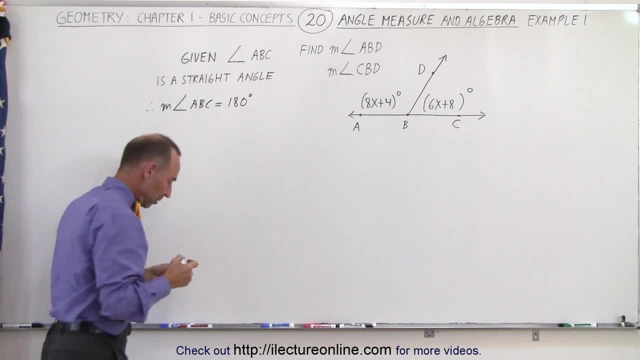 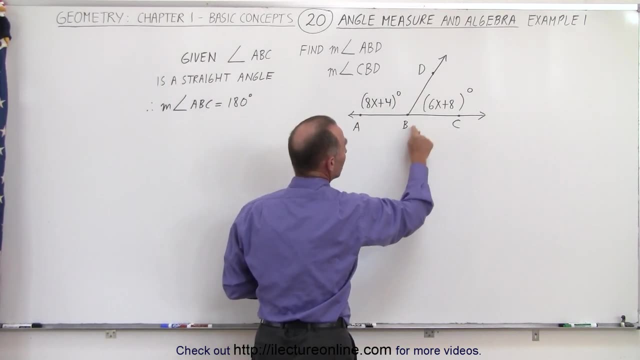 is 180 degrees. So that means that the measure of the angle ABC is 180 degrees is equal to 100 degrees, which then implies that the measure of the angle ABD plus the measure of the angle CBD together should add up to 180 degrees. so therefore we can say: 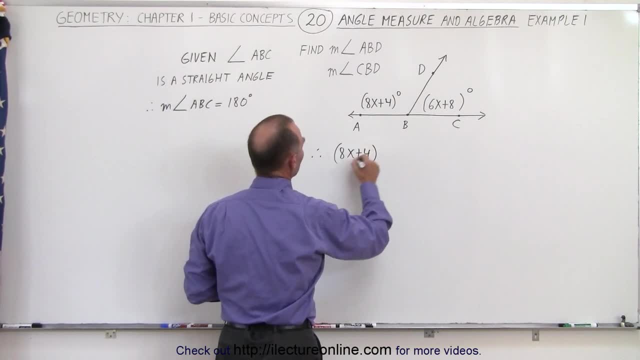 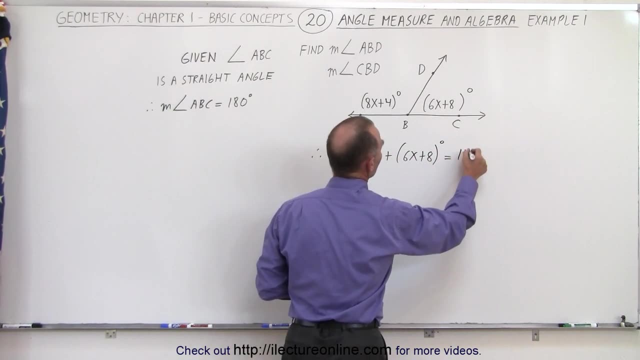 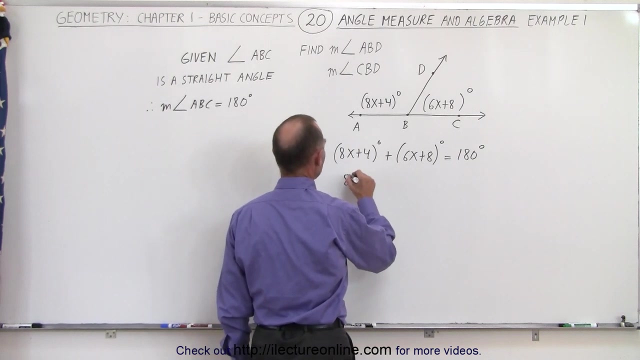 that 8x plus 4- and that would be in degrees plus 6x plus 8 in degrees, is equal to 180 degrees. To make things a little bit easier, we'll just go ahead and drop the degree notation, so we can say that 8x plus 4, added to 6x plus 8, must equal to 180, realizing that we're dealing. 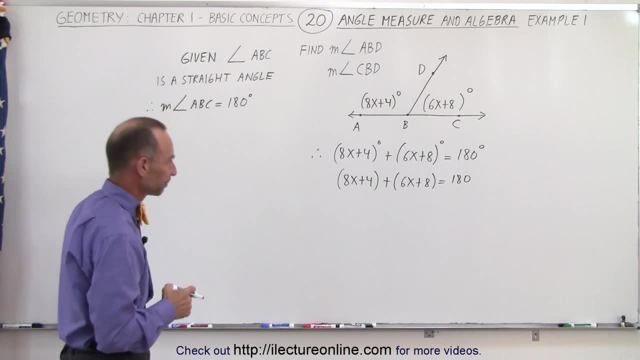 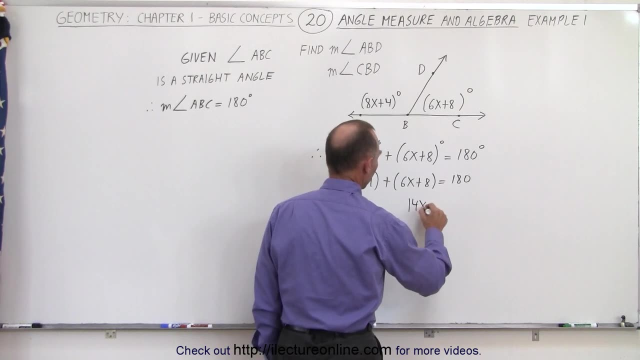 with degrees here. So now what we need to do is solve for x. On the left side, we have 8x plus 16x plus 6x. that's together 14x. On the right side, we have 180 minus 4x plus. 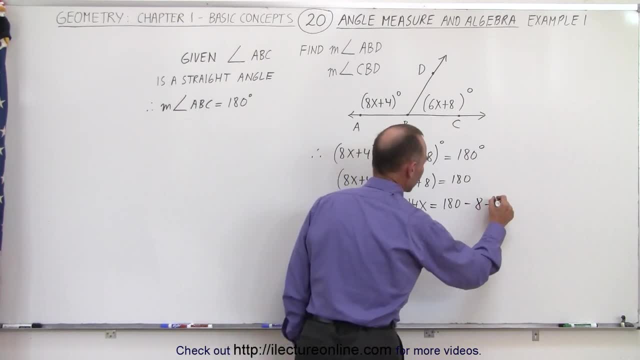 guidance: when we bring 8 across, becomes a minus 8, and let's bring the 4 across and get a minus 4.. That means that 14: x is equal to 180 minus 12 or 168.. Now, 10 times x is 140.